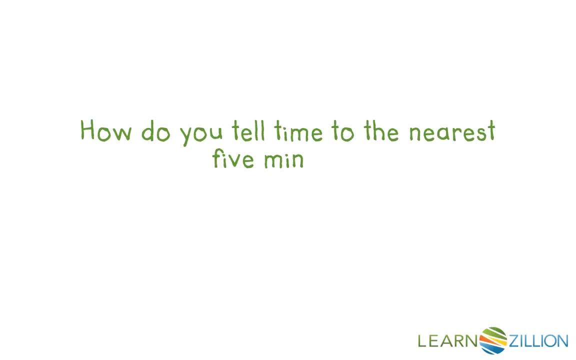 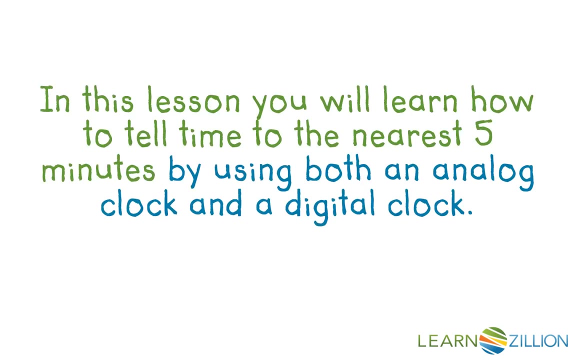 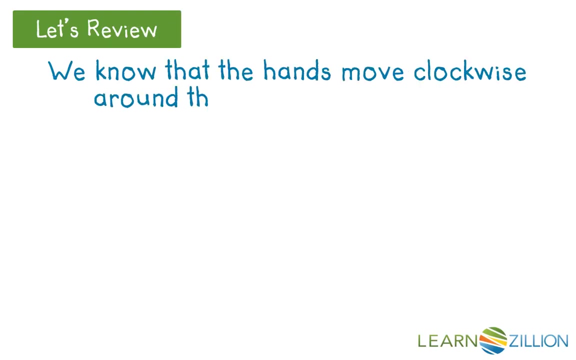 How do you tell time to the nearest five minutes? In this lesson, you will learn how to tell time to the nearest five minutes by telling time on both an analog clock and a digital clock. We know that the hands move clockwise around the clock as time passes. 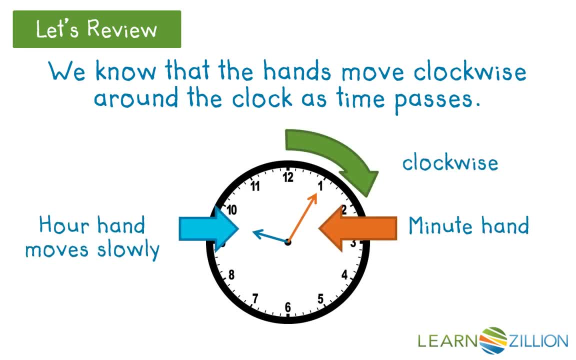 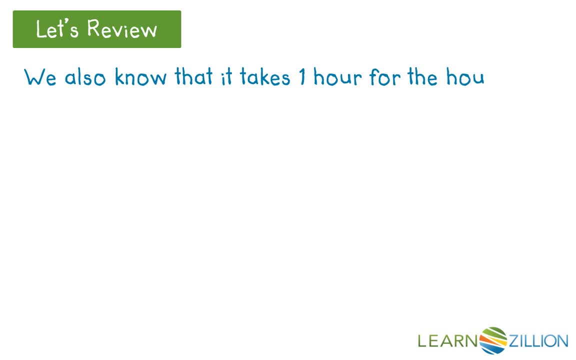 The hour hand moves slowly around the clock and the minute hand moves faster around the clock than the hour hand. We also know that it takes one hour for the hour hand to move from one number to the next and one hour or 60 minutes for the minute hand to move from the 12 all the way around the clock back to the 12 again. 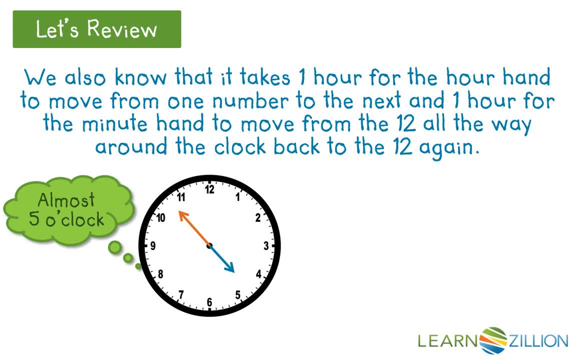 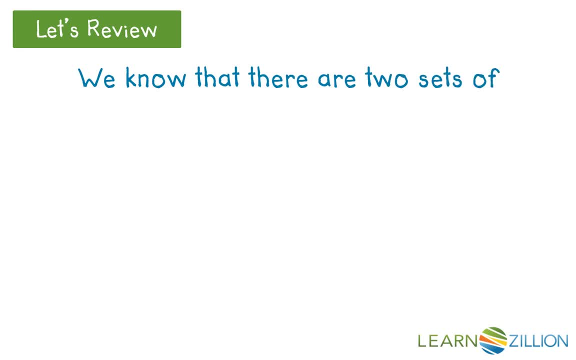 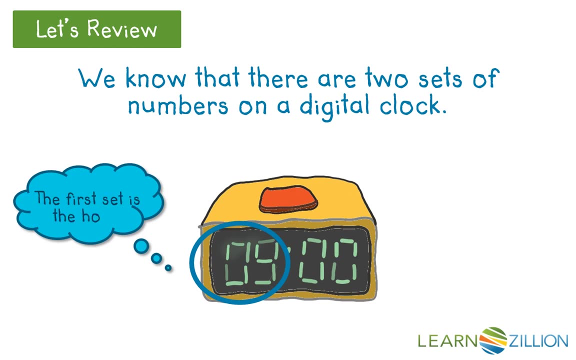 If the hour hand is between two numbers, the hour of the time is the number that is before the hour hand. We know that there are two sets of numbers on a digital clock. The first set of numbers is the hour of the time And the second set of numbers is the minutes past the hour. 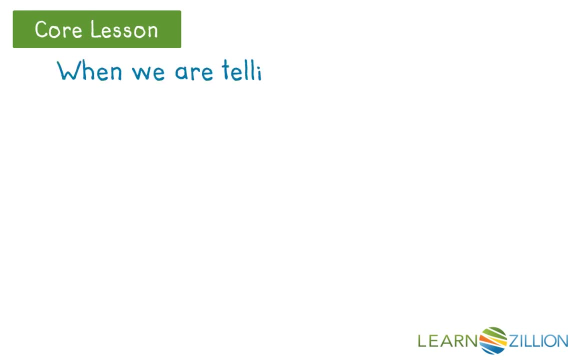 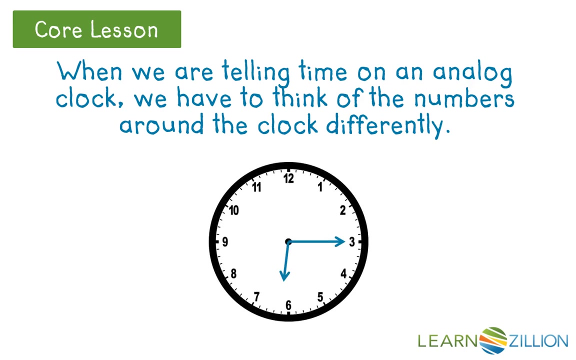 When we are telling time on an analog clock, we have to think of the numbers around the clock differently. The numbers on the clock really tell us what hour it is. When we are looking at how many minutes have passed, we know that the little tick marks represent each of the 60 minutes in one hour. 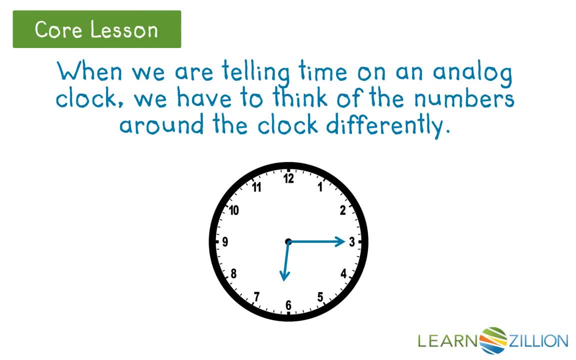 We can also count by fives, because there are five tick marks or minutes between each number on the clock. So if we look at this clock shown, the time is 615, because the hour hand is just past the 6 and the minute hand is on the 3,. 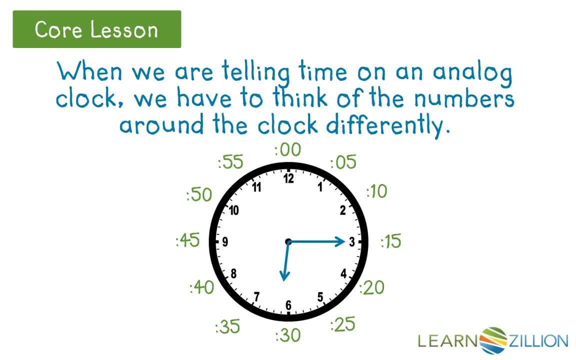 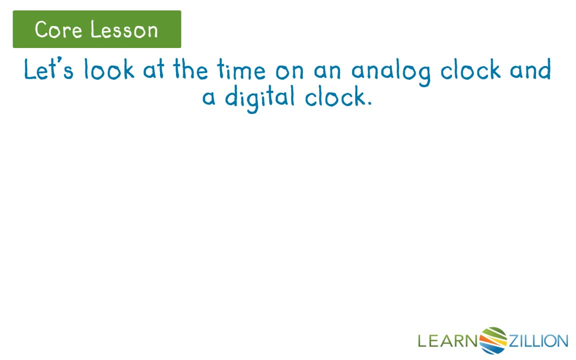 which means it is 15 minutes past the hour. Let's look at the time on an analog clock and a digital clock. On the analog clock, the hour hand is between the 3 and the 4, so we know that it is 3 something, because the hour hand is not to the 4 yet. 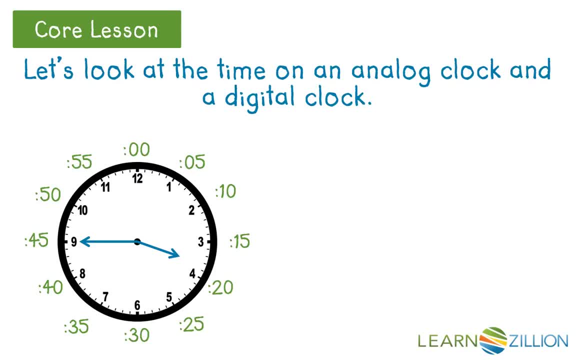 The minute hand is on the 9,, which is 45 minutes past the hour, because the minute hand began pointing directly at the top of the clock at the 12, when it was exactly 3 o'clock, and has moved 45 tick marks until it has gotten to the spot where it is. 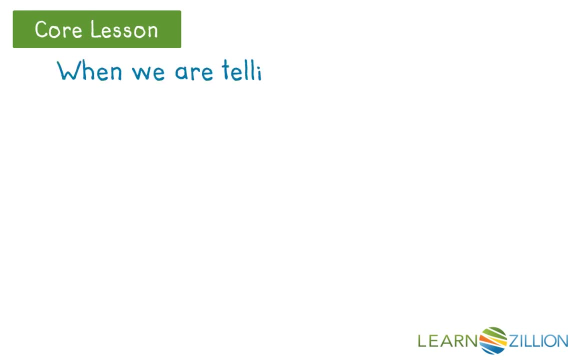 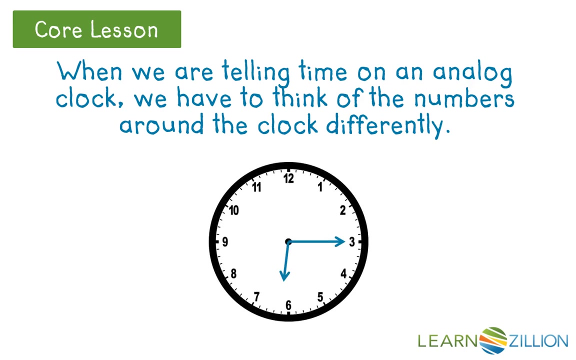 When we are telling time on an analog clock, we have to think of the numbers around the clock differently. The numbers on the clock really tell us what hour it is. When we are looking at how many minutes have passed, we know that the little tick marks represent each of the 60 minutes in one hour. 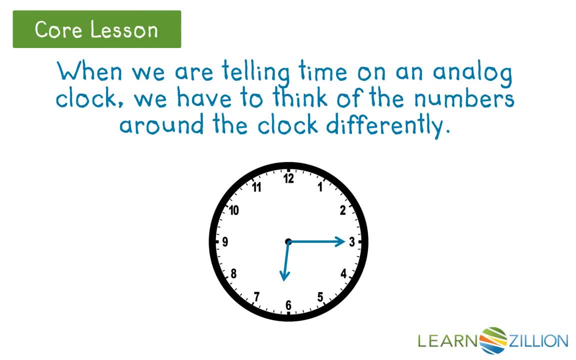 We can also count by fives, because there are five tick marks or minutes between each number on the clock. So if we look at this clock shown, the time is 615, because the hour hand is just past the 6 and the minute hand is on the 3,. 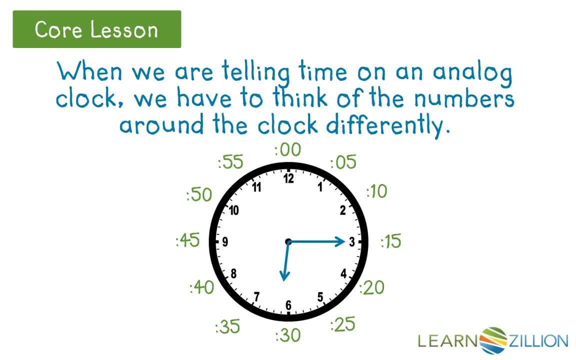 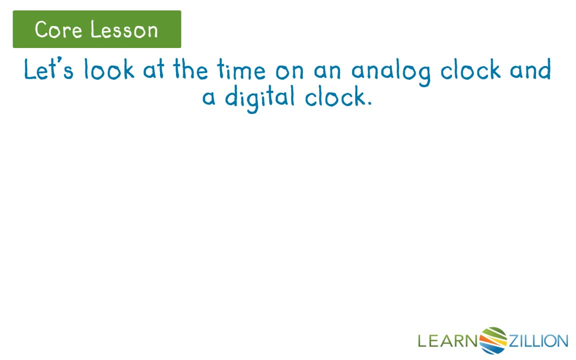 which means it is 15 minutes past the hour. Let's look at the time on an analog clock and a digital clock. On the analog clock, the hour hand is between the 3 and the 4, so we know that it is 3 something, because the hour hand is not to the 4 yet. 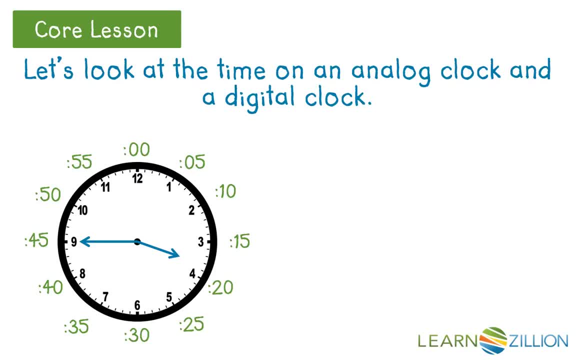 The minute hand is on the 9,, which is 45 minutes past the hour, because the minute hand began pointing directly at the top of the clock at the 12, when it was exactly 3 o'clock, and has moved 45 tick marks until it has gotten to the spot where it is. 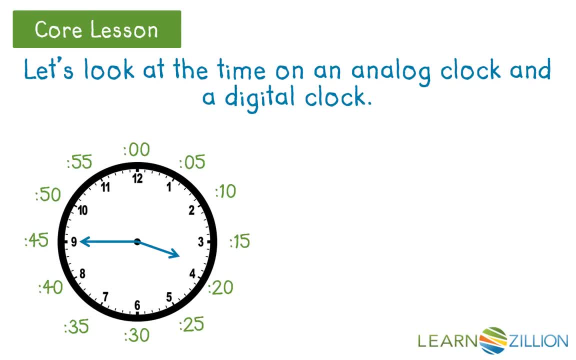 So the time on the analog clock is 345.. On the digital clock, the hour set of numbers is a 3. The minute set of numbers is 45. So the time on the digital clock is also 345.. This is the same time. 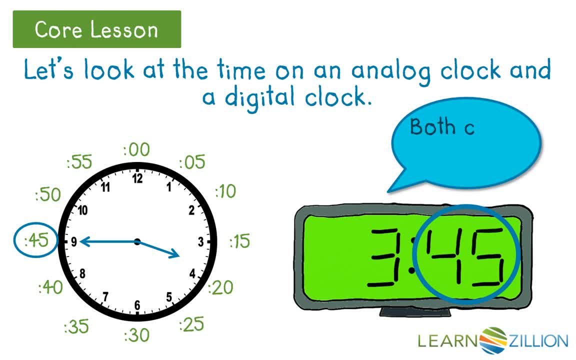 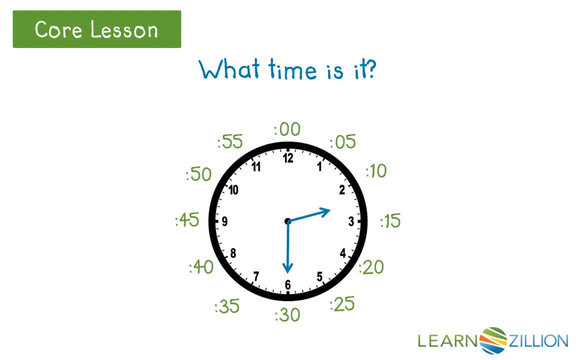 It is just shown on two different clocks What time is it? The hour hand is between the 2 and the 3, so we know it is 2 something. and the minute hand is on the 6, so we know it is 30 minutes past the hour. 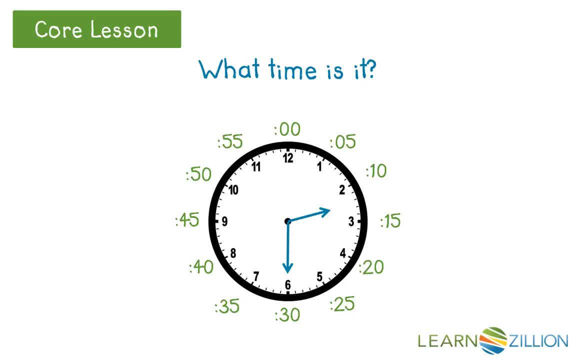 because the minute hand has moved 30 tick marks or minutes, since it was pointing directly at the 12 at 2 o'clock. so the time is 2.. So the time is 2.30.. What time is it? The hour hand is between the 4 and the 5,. 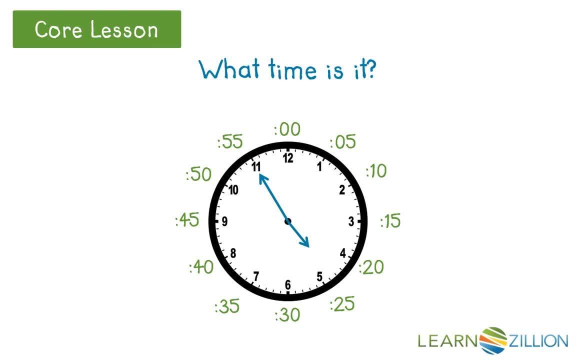 so we know it is 4 something and the minute hand is on the 11,. so we know it is 55 minutes past the hour because the minute hand has moved 55 tick marks since it was pointing directly at the 12 and it was 4 o'clock.